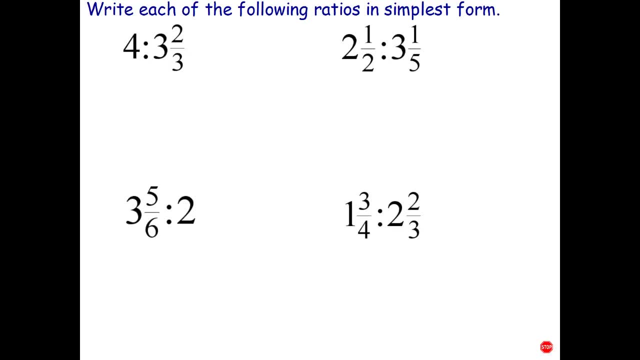 Hello students, In this video we are going to show you how to simplify two numbers where at least one of the numbers is a mixed number. So let's have a look at this question up here. Four is to three and two thirds. Well, to start with we're going to write each of these as a fraction, So four we write as four over one, Three and two thirds. Well, three times three is nine plus two is eleven, So that 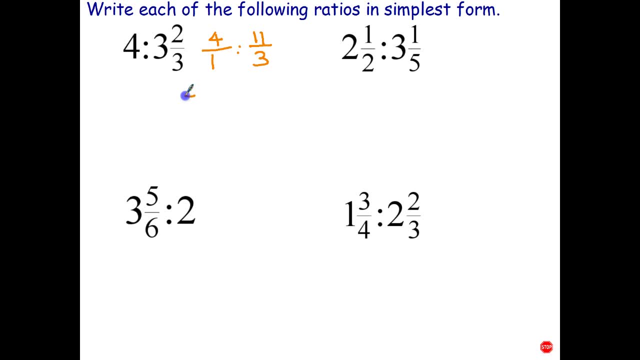 becomes eleven thirds. The next step is to then get a common denominator. So in this case the common denominator will be three. So the eleven over three just stays the same. And here I think one times three is three, Four times three is twelve. So I just rewrote that with a new denominator of three. And finally, because the denominators are the same, we can: 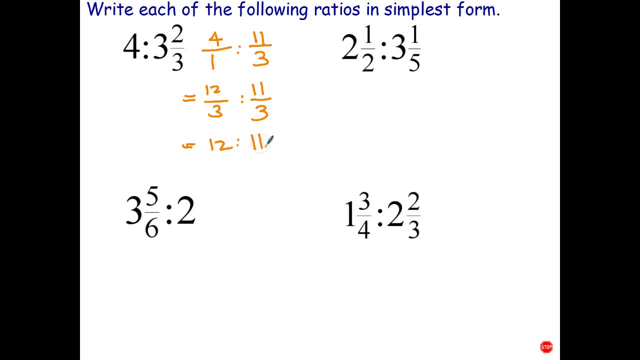 rewrite that as just twelve is two, eleven, And that's in simplest form. So that's as far as we need to go. Okay, why don't you have a go at the remaining three questions and then restart the video and see how you went? Okay, let's have a go at this question here. Two and a half is to, three is three and one fifth. So to start with, we write each of these as an. 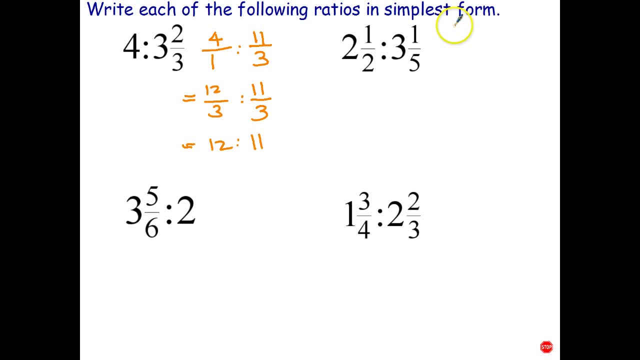 improper fraction. So two times two is four plus one is five, So that's going to be five over two. Five times three is fifteen plus one is sixteen, So that's going to be sixteen is to five. Okay, now we have to find the common denominator. So we have two and five. Common denominator is ten. So we'll write each of those with a base of ten. 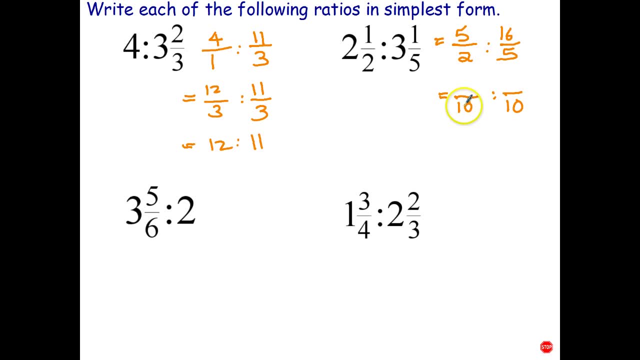 or denominator of 10. 2 times 5 is 10. 5 times 5 is 25. 5 times 2 is 10. 16 times 2 is 32. now that we have a common denominator, we can rewrite the ratio just using the numerators. so we have 25 is. 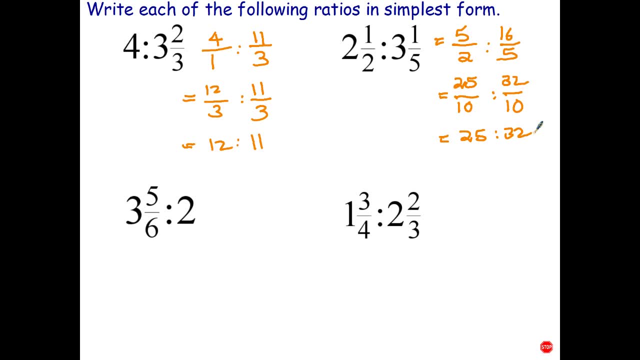 232, and once again they cannot be simplified. so that's the final, that's already simplified, I should say. so that's the final answer. third question: write the first number as an improper fraction: 6 times 3 is 18 plus 5 is 23 over 6, and the second one we just write is 2 over 1 any whole. 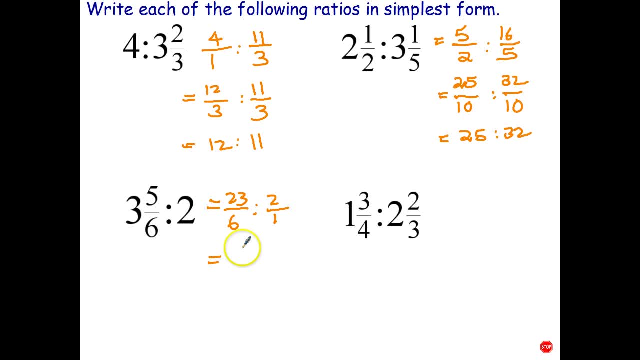 number can be written with 1 and the denominator, so 6 is going to be our common denominator. 23 on 6 stays the same: one times 6 is 6, 2 times 6 is 12 and again because the denominators are the 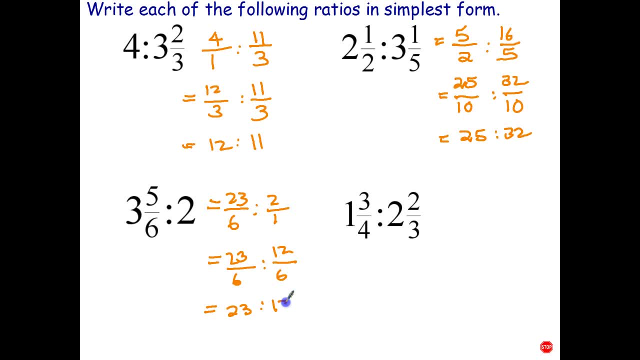 same. we can just write that as the ratio of the numerators and once again, that's already simplified, so we can just hours or degrees with that in mind. so let's do that. subscribe to my. we don't need to go any further on that one. okay, the last question, right one in: 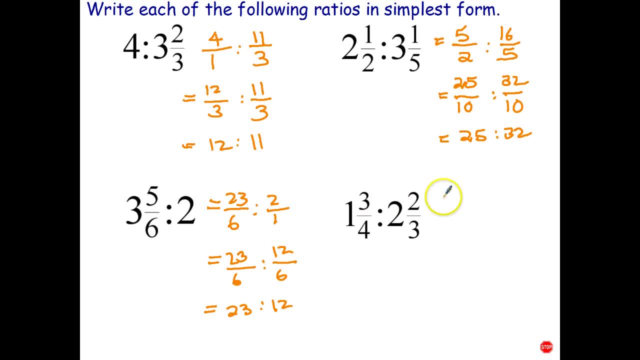 three quarters, as 4 times 1 is 4 plus 3 is 7, so that becomes 7 over 4. 2 times 3 is 6 plus 2 is 8, so that becomes 8 over 3. okay, we now need to get a common. 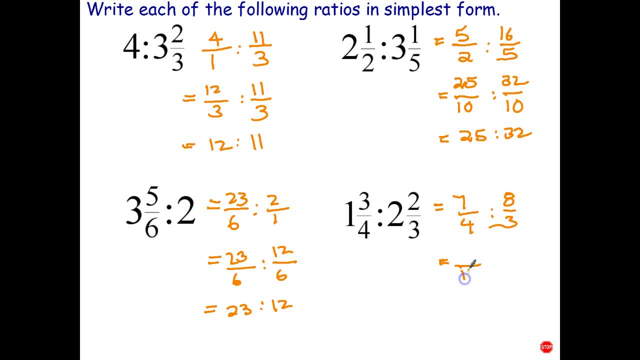 denominator. well, the common denominator of 4 and 3 is 12. 4 times 3 is 12. 7 times 3 is 21. 3 times 4 is 12. 8 times 3. 3 times 4 is 12. 8 times 4 is 32. so once. 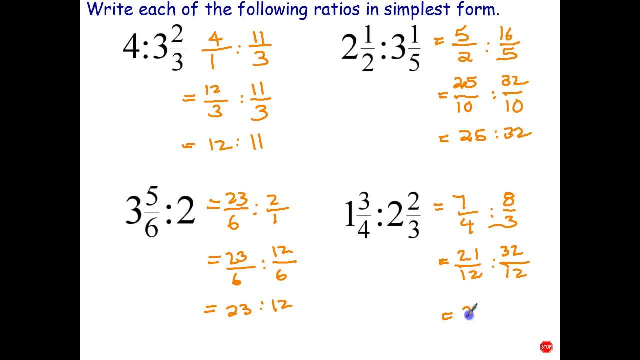 again, the denominators are the same. oops, let me just undo that you get rid of that ugly looking. equal sign denominators are the same, so we can equate the numerators or just compare the numerators: 21 is to 32 and once again there's no common factor. so that's the final answer.